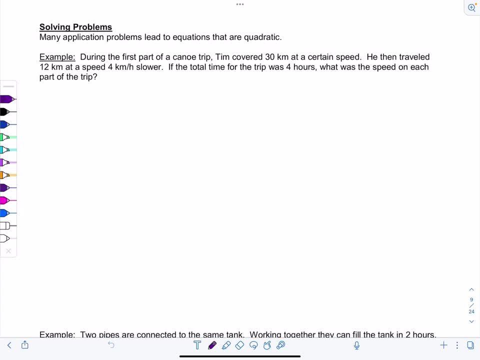 solve quadratic equations. I recommend you do that before you dive on ahead. But here we're just going to start setting up word problems. The setup is definitely the hardest part for most students, So let's jump to it. First example: During the first part of a canoe trip. 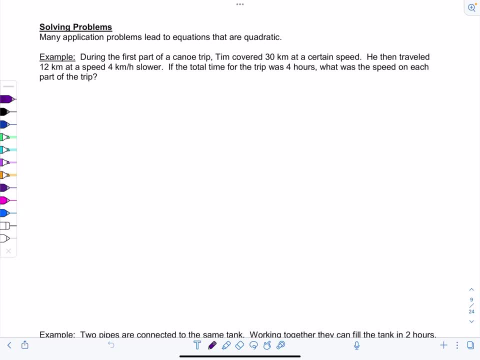 Tim covered 30 kilometers at a certain speed. He then traveled 12 kilometers at a speed four kilometers per hour slower. If the total time for the trip was four hours, what was the speed on each part of the trip? So anytime you have these motion problems, 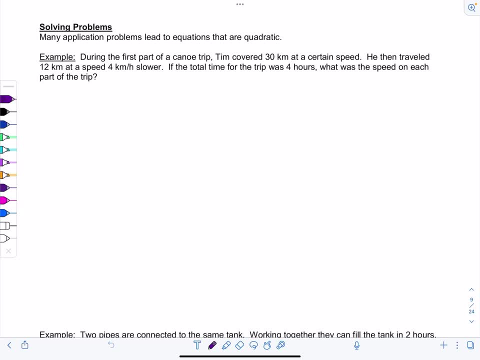 I like to call them, whether it's little Timmy canoeing or someone flying an airplane or rowing in a river, et cetera, et cetera. you're going to use distance, equals rate, times, time, And then we're going to: let's set up a table. I think that's the best way to do it, to summarize all. 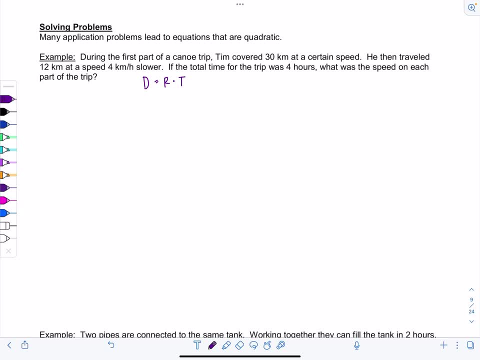 the information that we're given And then, after you've done that, you're going to go to the table. We can see. okay, how can I write an equation using all of this that I'm going to solve and answer the question with? So notice, here there's two parts of the trip. He has a. 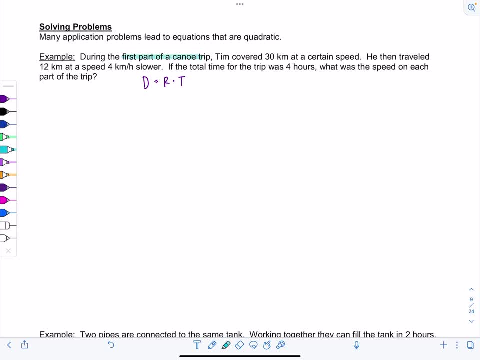 first part of a trip, and then there's a second part of the trip where he's slowing down. Maybe his little arms got so tired, poor thing. So two parts to the trip. What does that mean? I'm going to have two rows in my table, So distance equals rate, times, time, And then I'm going to go to the 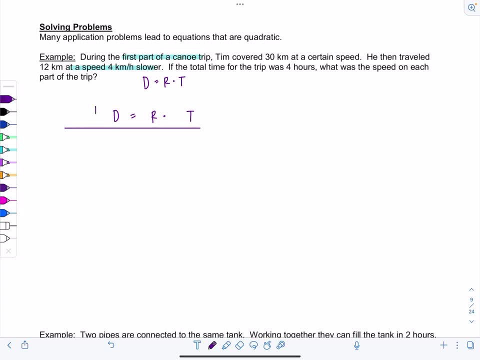 first part of the trip. So distance equals rate, times, time. Those are pretty much the columns, Okay, And then we have part one of the trip and we have part two. So those are our two rows, And then let's fill in the information that we have in the word problem. Okay, So let's see. 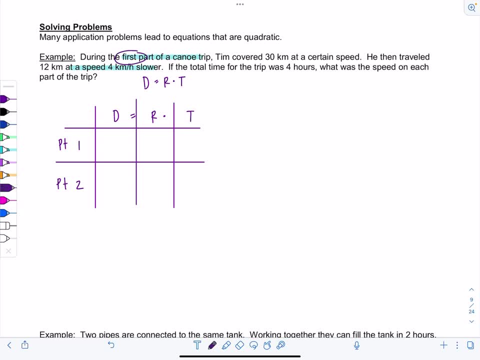 In the first part of the trip he covered 30 kilometers. That's the distance for part one. So please put a 30 right here for the distance At a certain speed. I don't know the speed. Okay, Time to bust out a variable. I'm going to call. 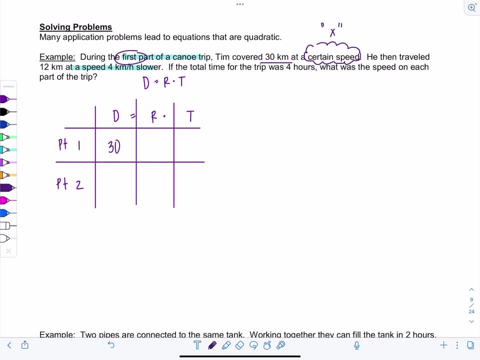 that speed. X. Don't get too fancy schmancy and try to use S or stuff like that. I think it just messes with your brain. Okay, X. They didn't say anything about the time, Did they No? So this is. 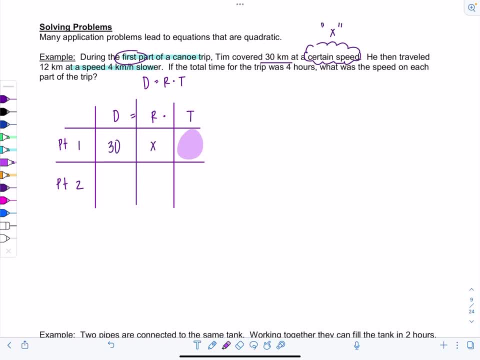 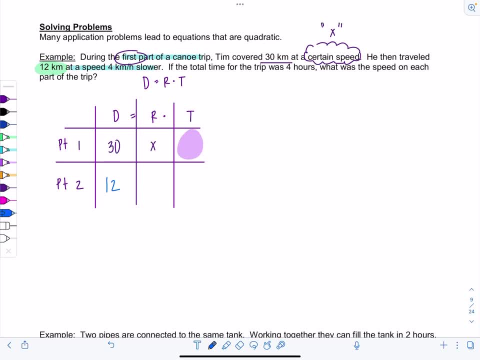 part two of the trip. Okay, Watch this At a speed four kilometers per hour slower, slower than X. So make sure you get the order of subtraction right. Four kilometers per hour slower is four less than X. That's going to be X minus four, not the other way around, And just think about it. 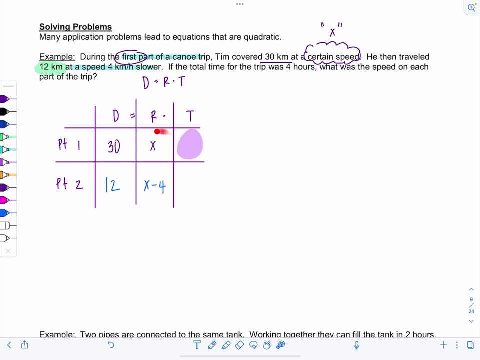 Think what makes sense in your head. Say he was going 10 kilometers per hour Originally. what's four? slower, It's six. How did you get there? 10 minus four, Not the other way around? Not four minus 10.. When you're doing subtraction, the order is super important that. 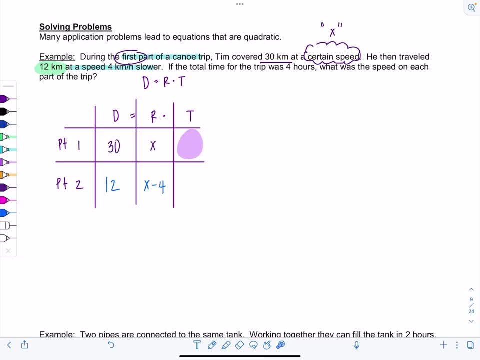 you get it right, Otherwise it will mess up the entire problem. Okay, Do they say anything about the time on part two? No, they don't. But what do they tell us? They tell us the total time for the trip was four hours. Hmm, That's the total time. Total time would be the time from part two to part two. 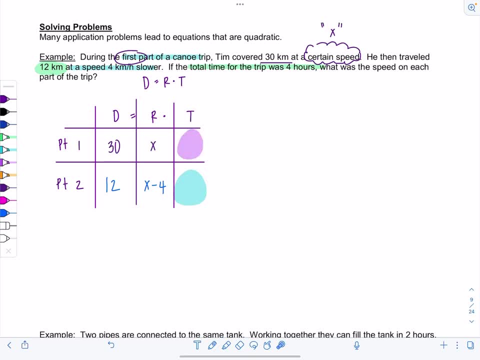 Part one plus the time for part two, That should be four hours. So here's the thing. Resist the urge to bust out a second variable. It's unnecessary. Okay, If you're doing a quadratic equation, you've got to stick to just one, especially if you're in algebra. So how am I going to fill in? 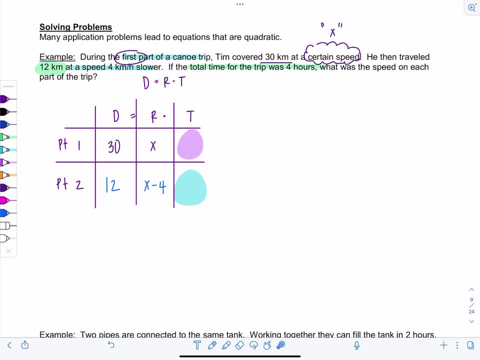 those entries for time on part one and part two. Watch this: If we know distance equals rate, times time- and I'm missing time- isolate T in this equation. So distance divided by rate equals time, Do you agree? Oh good, So that means the time for part. 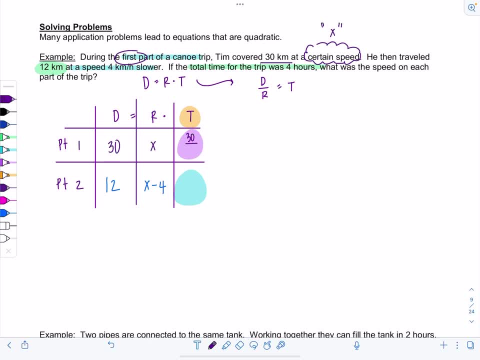 one is going to be the distance covered in part one: 30, divided by the rate in part one, which was X, And then similarly for part two. the time for part two is going to be the distance: 12, divided by X minus four. Good, Now, how do I write an equation using this table That will: 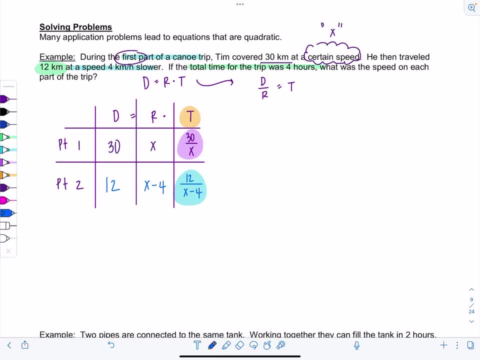 be different. I'm going to use this table. I'm going to use this table. I'm going to use this table For every single word problem. In this particular case, they told me that the total time for the trip was four hours, So that means the sum of the time for part one and part two should equal four. 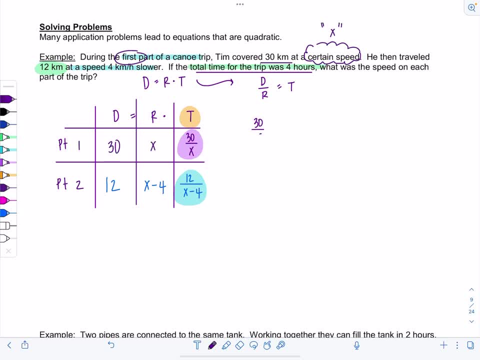 So here's my equation: 30 over X plus 12 over X minus four equals four. right, That's the sum of the time for part one and part two. Now, this is a rational equation And we've studied these before. When we solve, we want to. 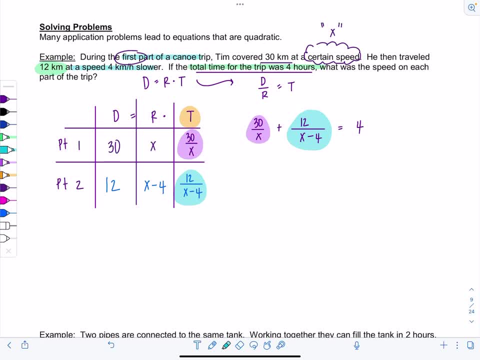 make sure. first we list the domain And then we're going to clear out all of the fractions. We don't want anything in the denominators by multiplying through by the LCD So domain, remember. you don't want any zeros in the denominator. That means from this guy X cannot be zero. And also here. 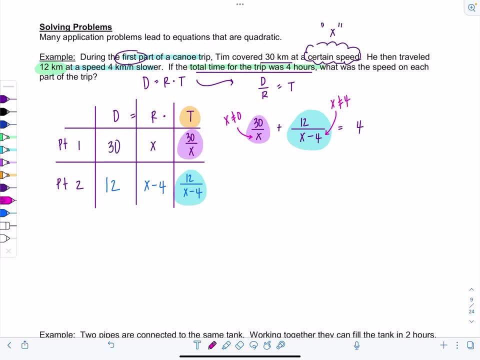 X cannot be four. Okay, So those are our two restrictions. Now we have to multiply the equation through by the least common denominator, least common multiple same thing. in this case, it's going to be X times X minus four the goal. 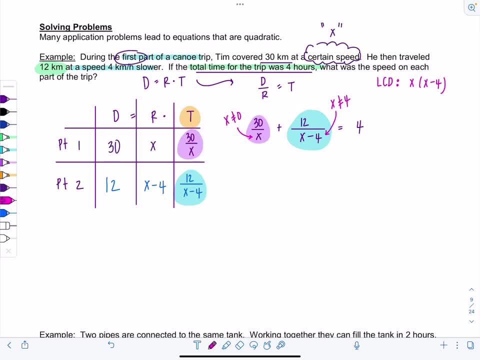 is to be fraction free, Okay. So I'm going to multiply everybody by X and X minus four. Okay, And if you need to actually write it out and distribute, go for it. I'm not going to because it's just going to be a fraction free, So I'm going to multiply everybody by X and X minus four. 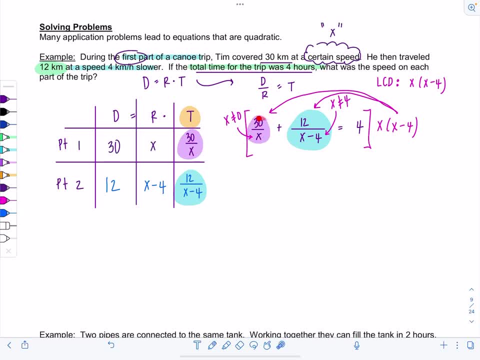 So I'm going to do it mentally. If I have 30 divided by X times X and X minus four, this X will cancel out with the X in the denominator. So all I'm going to be left with is 30 times X minus four plus 12.. Now notice in this case, when this distributes to 12 over X. 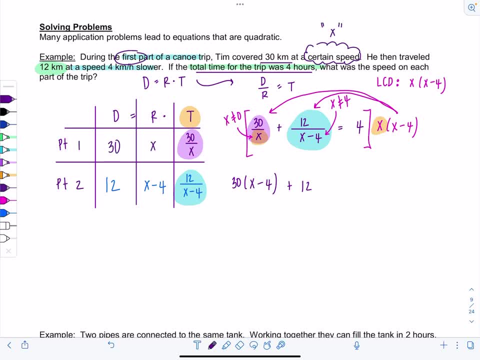 minus four. the X minus four will cancel. So I just have 12 times X left And then nothing cancels out. So I'm going to do it mentally. If I have 30 divided by X times X minus four, it cancels on the right. So you've got four X times X minus four. 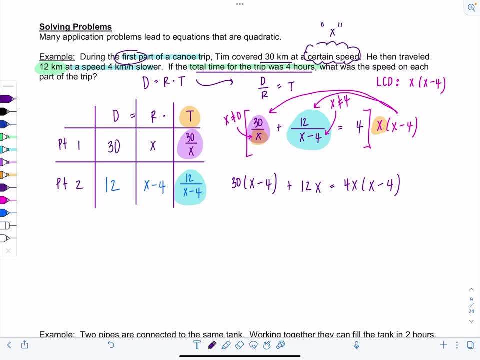 All right, Looks good, Let's distribute. I mean, it's looking better, There's no fractions. We should be excited. So this is 30 X minus 120 plus 12 X equals four X squared minus 16 X. As soon as I notice: oh, I got a quadratic equation. quadratic because there's that X. 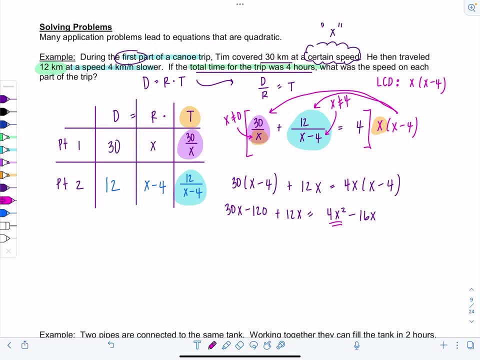 squared term. Let's set it equal to zero And then we'll decide from there. can we factor or do we quadratic formula? Okay, So I'm setting everything to zero. Before that, let's clean up. This is: 42 X minus 120 equals four X squared minus 16 X. So I'm going to subtract 42 X and add 120.. That way, 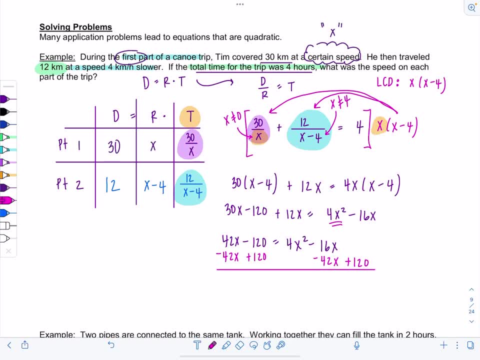 I have a zero on one side. It doesn't have to be the right side, Okay. Whichever side is nicer. I want a zero on the left because I like to keep the X squared term positive. Okay, So now we have zero equals four X squared minus 58, X plus 120.. Now, before I try to factor, 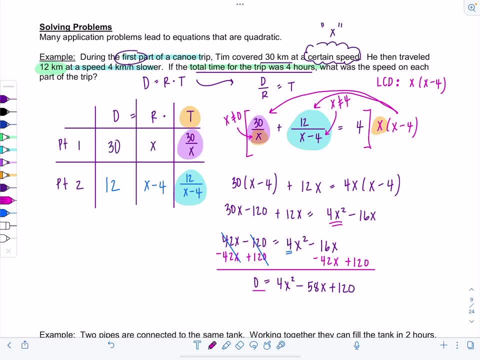 or do the quadratic formula. I noticed I can divide everything by two, So let's go ahead and do that. Okay, Okay, Professor V. good, So we have. zero equals two X squared minus 29, X plus 60.. Okay, Good, So it's up to us. Let's see if this factors And if it's giving us too much of a. 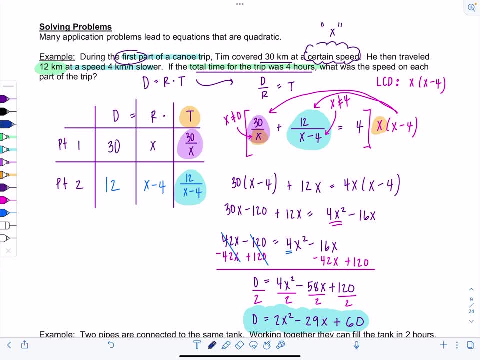 headache. we can do the quadratic formula. I've shown in a video before how you can do splitting the middle term with the AC method. So you put A times C up top, So A is two and C is 60. So A times C is 120. And then B goes in the bottom, which is negative 29.. 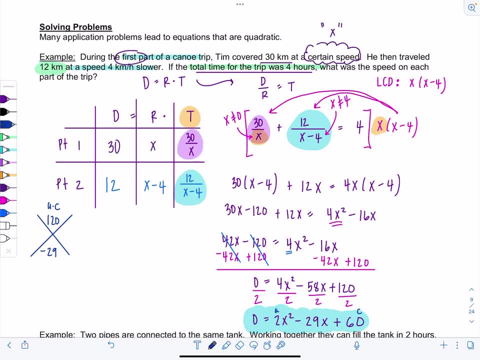 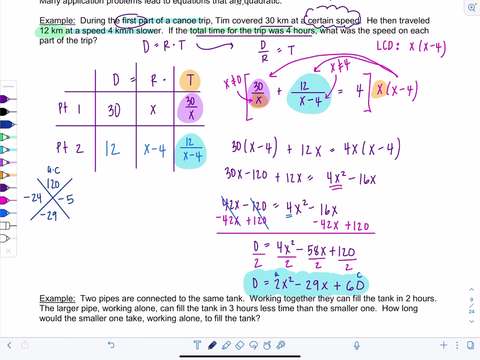 So can you think of two numbers that multiply to 120, but add to negative 29? And it's negative 24 and negative five, right? Negative 24 times negative five is 120. And they add to negative 29.. So what I'm going to do is now split the middle term, So I have two X squared minus 24 X. 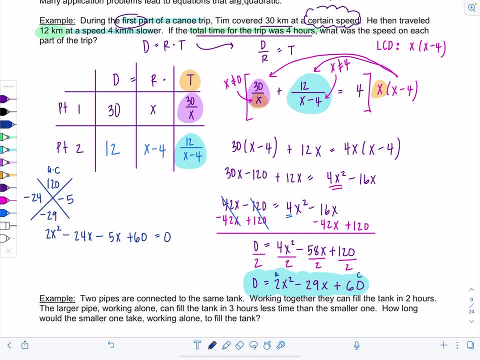 minus five. X plus 60 equals zero. Let's take out the greatest common factor here, That's a two X, And then we have X minus 12.. Here I can take out minus five, And then we have X minus 12 is zero. 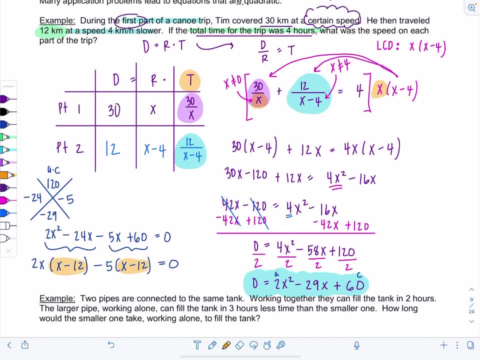 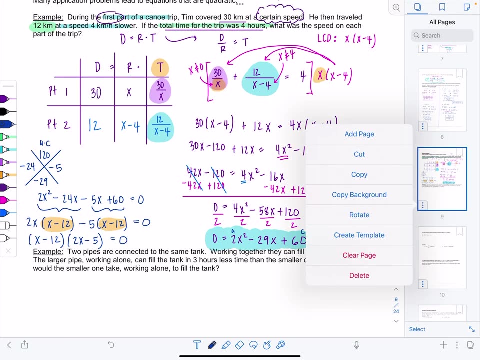 And then look at X minus 12,, X minus 12.. I can factor that out, And then you have two. X minus five equals zero. Okay, now from here. you know I need more space. It is what it is. Okay, So from here. 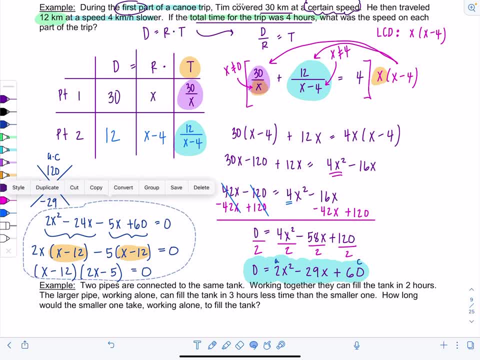 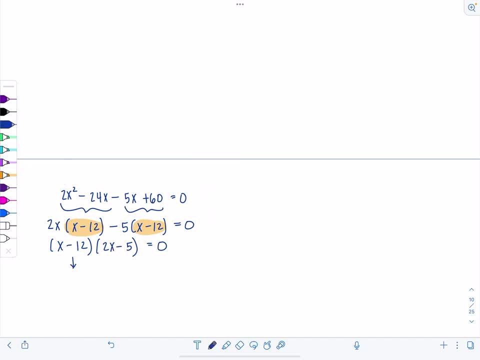 let me copy all of this And let's go down here. We'll return momentarily From here. you're going to use the zero product property, set each factor equal to zero And then solve for X. So X is either 12,. 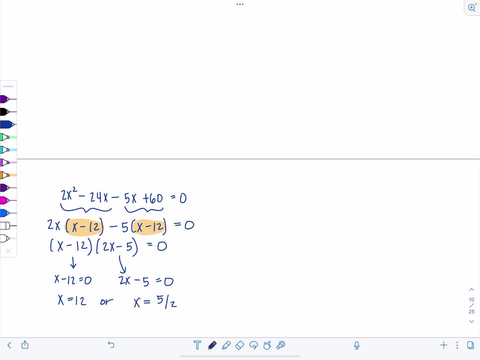 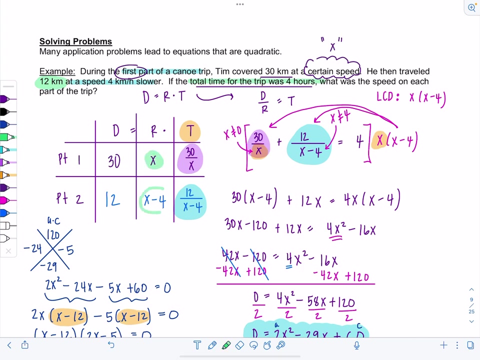 or X is five halves Now both of them won't work. So in a word, problem. you have to think like what's going to make sense. X is the speed on the first part of the trip, Okay, And then X minus four is the speed on the second part of the trip. 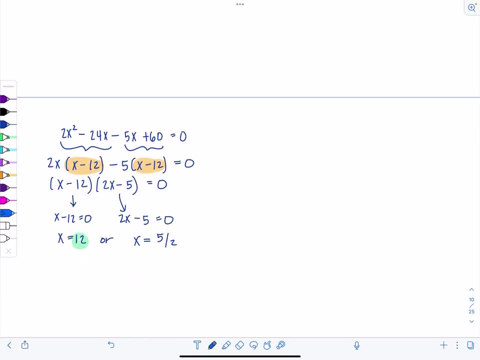 So if X is 12, that would mean he's going 12 kilometers per hour on part one, And then four less than that would be eight kilometers Per hour, which makes sense. If X is five halves, that's 2.5, right as a decimal. 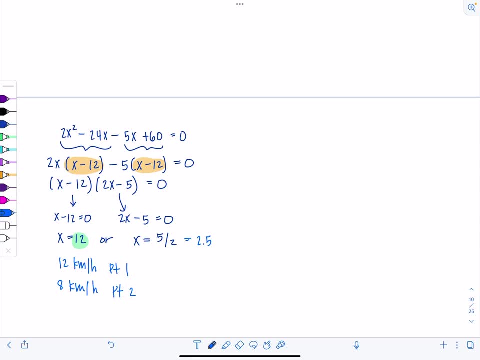 So if he's going 2.5 kilometers per hour on the first part of the trip, he can't go four kilometers per hour slower than that. It would be negative. So I can tell: oh, this one doesn't make sense, I'm throwing this one away. Okay, So here's the answer to. 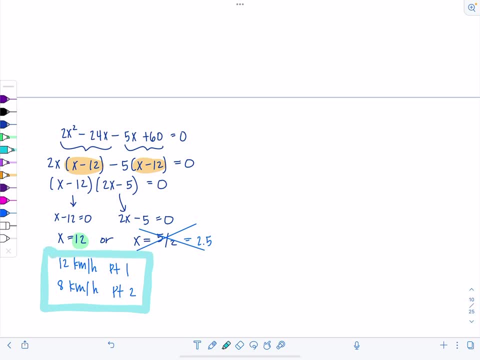 the problem. This gives us the speed on each part of the trip. Okay, But I know what you're thinking. You're thinking, oh my goodness, Professor V, It was kind of aggressive. to factor 2X squared minus 29X plus 60 equals zero. Like, how did you come up with negative 24 and negative five to? 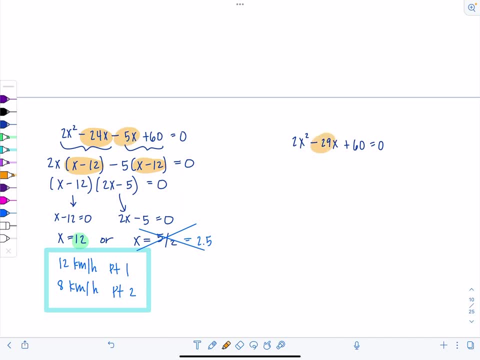 split the negative 29?? Yes, I am a factoring queen. I know I've done this for a long time. If you're still struggling and that's just too tricky of a way to solve it, then you can use the quadratic formula, Okay. 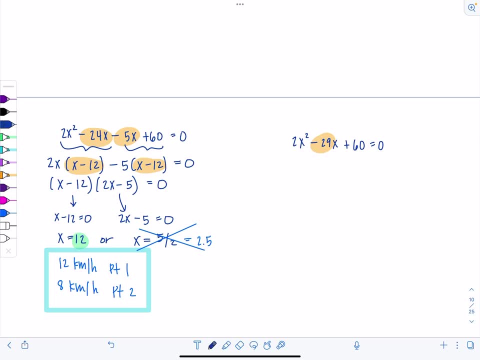 So it's nice, Let's review because it's helpful for situations where the factoring might be a little hard. Let's write out the quadratic formula: X equals opposite of B, plus or minus square root. B squared minus 4AC all over 2A. And then here's A, B and C. right A is 2,. 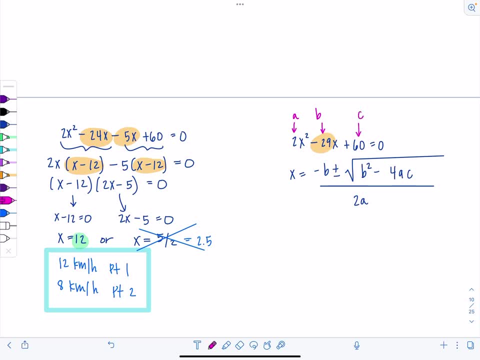 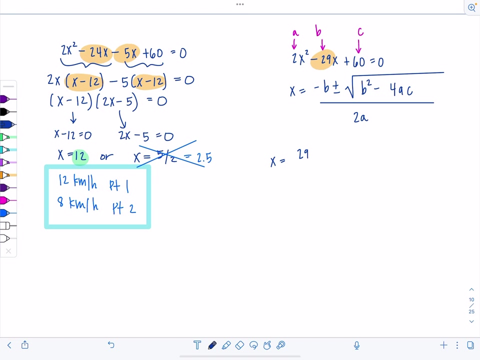 B is negative 29, and C is 60. Okay, The only thing is, with these big numbers the computation is going to get a little tricky, So make sure you keep your skills sharp. I don't know if your instructor lets you have a calculator or not. So opposite of B is going to be positive. 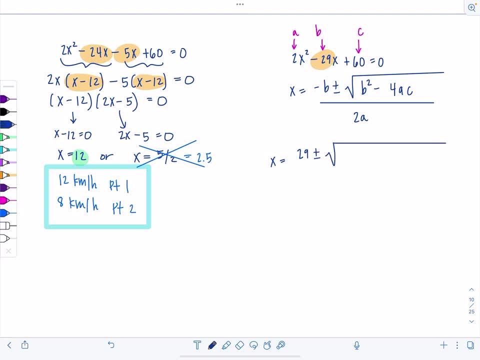 29 plus or minus square root B squared, That's negative. 29 squared minus 4 times 2 times 60, all over 2 times 2.. So this is 29 plus or minus square root 441.. That's negative 29 squared. The negative goes away. Minus 4 times 2 is 8 times 60, 480. 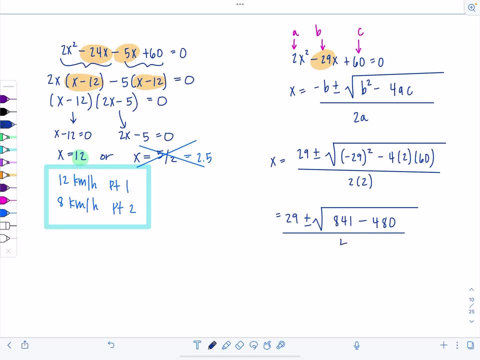 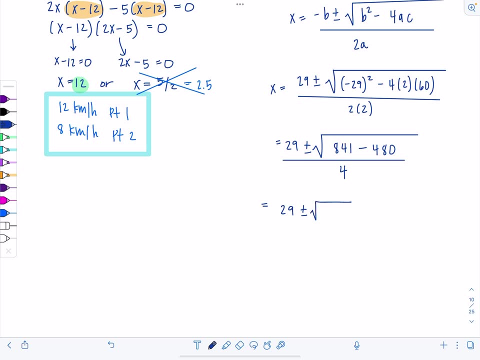 over 2 times 2 is 4.. And then this is going to be 29 plus or minus square root of 361 over 4, which is 29 plus or minus 19 over 4.. So how do you proceed from here? 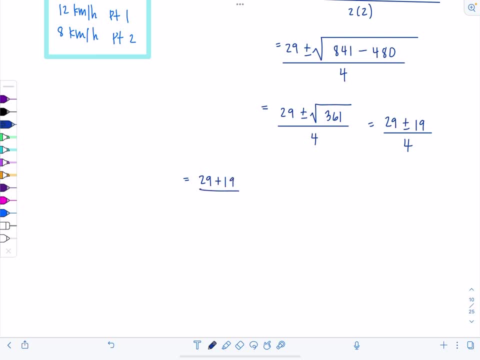 Well, you do 29 plus 19 over 4, or 29 minus 19 over 4.. You've got to separate them at this point. 29 plus 19 over 4, that is 48 over 4, which is 12.. Or 29 minus 19,, that's 10 over 4,. 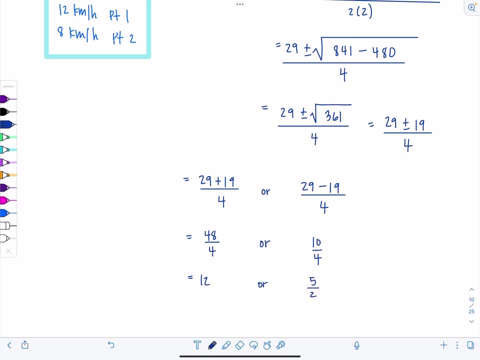 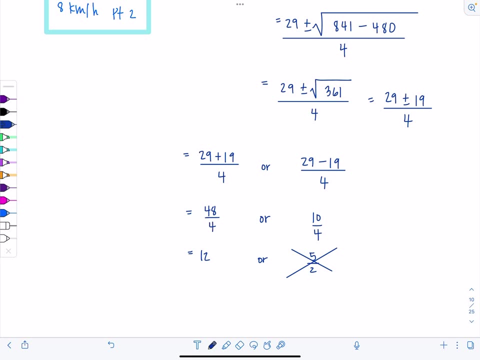 which is 5 halves, And those are the same answers we got when we factored, And then we knew to throw away this And we kept 12 kilometers per hour, Okay. The question did ask, though: what was the speed on? 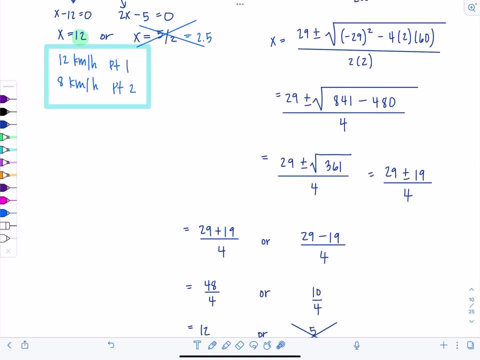 each part of the trip. So make sure when you answer the question you say 12 kilometers per hour for part one, and then 12 minus 4, which was 8 kilometers per hour for part two. Okay, Good, All right, Let's look at the next example. This is a work problem. We've done some before. 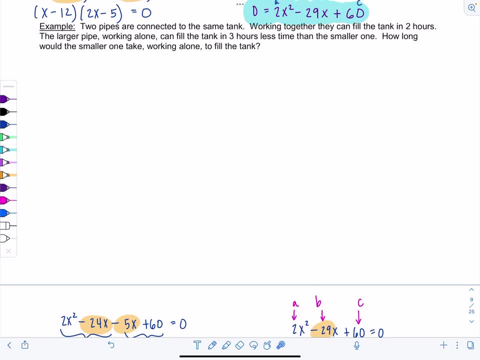 in previous video lectures. So the setup's going to be the same, It's just this time it's going to be a quadratic equation to solve. So two pipes are connected to the same tank. Working together, they can fill the tank in two hours. The larger pipe, working alone, can fill 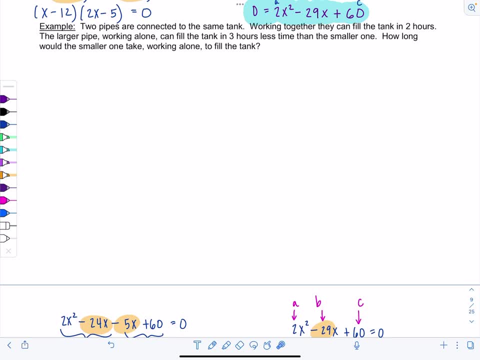 the tank in three hours- less time than the smaller one. Okay, How long would the smaller one take working alone to fill the tank? So I know these are so gnarly. when you read them They sound terrible, but they're actually not that. 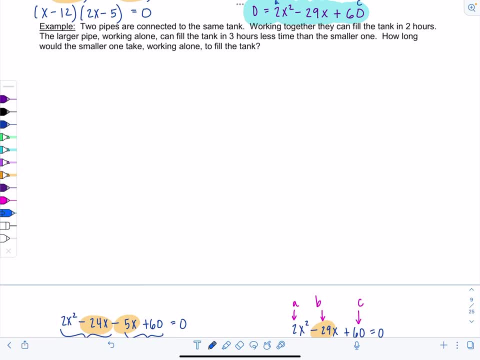 bad once you see the pattern to them. Always let your variable represent the quantity that you have the least information about. What do I mean when I say that? Okay, So they're telling me right here? this is the sentence. the larger pipe working alone can fill the tank in three hours less than. 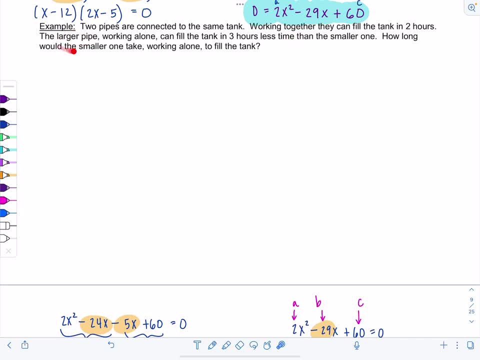 the smaller one. So they're telling me all this stuff about the larger pipe. They didn't tell me anything about the smaller one. And then the question says: how long would the smaller one take working alone to fill the tank? So that's what I'm going to: let my variable be. So I'm 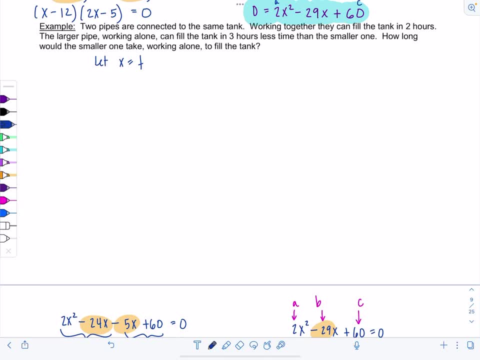 going to let x be the time it takes for the smaller pipe to fill the tank. Okay, And then if the larger pipe takes three hours less time, then that means the smaller pipe can fill the tank in three hours less than the smaller one. 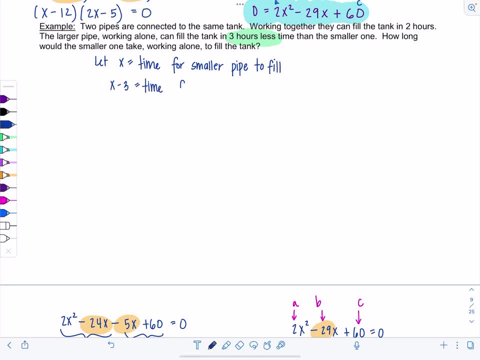 So that means x minus three would be the time for the larger pipe to fill the tank. Do you see how that works? Okay, So let your variable represent the quantity that you have the least information about. Okay, So in one hour let's see what equation we can write. You always do it in one. 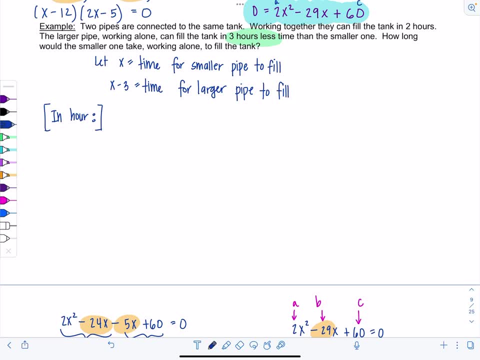 unit of time. Okay, So if the smaller pipe takes x hours, after one hour goes by it has filled up one over x of the tank. What do I mean by that? Okay, Think about it. Pretend we had a number for this. 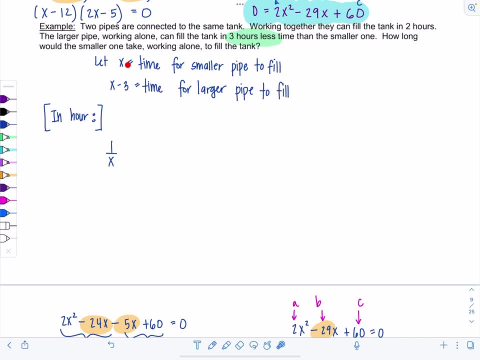 Pretend it takes five hours for the small pipe to fill the tank. Five hours, I'm just saying pretend, Just pretend. Okay, Five hours. If only one hour goes by, what fraction of the job is done? One fifth of it, Right. Or say it takes two hours After one hour half of it is done, So one over the. 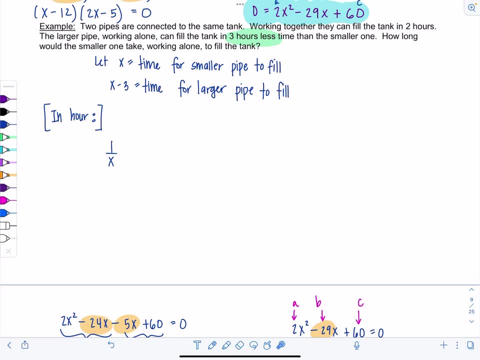 time is the fraction of the total job that is completed. Okay, So in one hour one over x is filled from the small pipe, Plus how much has the large pipe contributed? One over x minus three, And it told me it takes two hours when they work together. 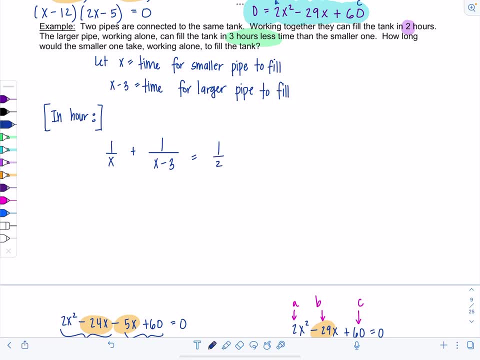 So after one hour, how much is done? One half, It's always one over the time, One over the time, One over the time. Do you see that? Here's our equation. That's it. We didn't have to make a. 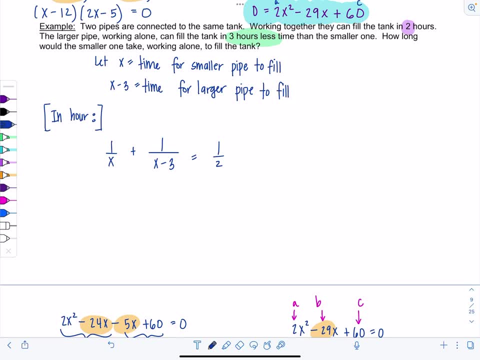 table. Do you hate it? Don't hate it, Just practice and you'll love it. Okay, Let's list our domain. So x cannot be zero or three, And then now I'm going to multiply everybody by the LCD. Let me. 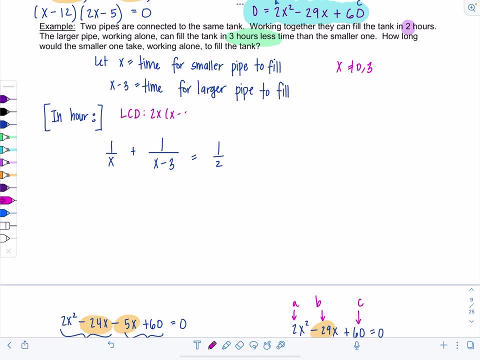 write it out here. The LCD is two x Times x minus three. If you are struggling with that step, then you need to review solving rational equations. I'll link that video here. So you multiply by the LCD in the numerator like this: Two x x minus three, Two x x minus three. This is the step I didn't show earlier because 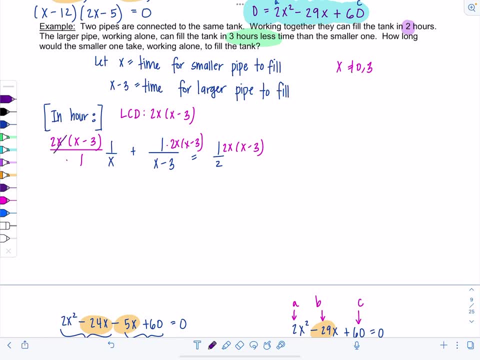 it's a little cumbersome. Okay, look, And then here this x cancels. So then you just have two times x minus three plus Then the x, x minus three cancels. So this is two x, Then the two cancels here, So it's x, x minus three. 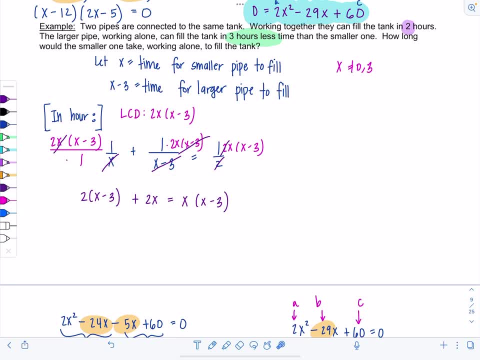 Okay, So in the last problem I didn't write this all out. You can do it in your head, No problem. Okay, Let's clean up here. See, we're fraction free. So two x minus six plus two x is x squared minus three x. So we have four x minus six equals x squared minus three x. We. 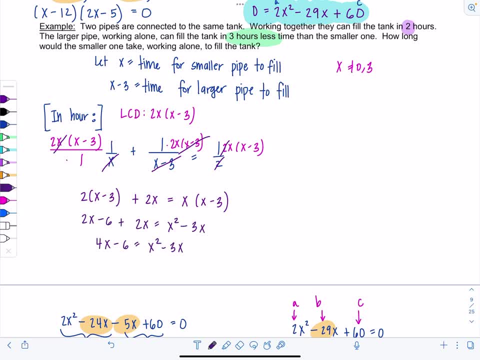 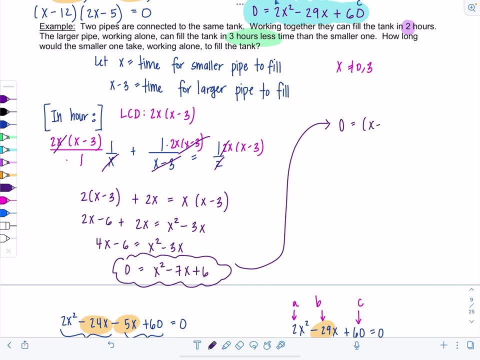 this No big deal. Zero equals x minus six, x minus one. I love it. So x is either six or one. One of these doesn't make sense and we got to throw it away. Which one? Okay, Yep, One. 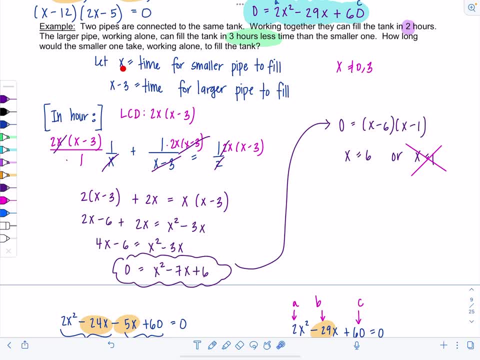 Why does that one make no sense? Because if x is one, one minus three would be negative two. That wouldn't make sense for the time for the larger pipe to fill. Okay, So let's see. Can we answer the question: How long would the smaller one take working alone to fill the tank? Yes, The smaller. 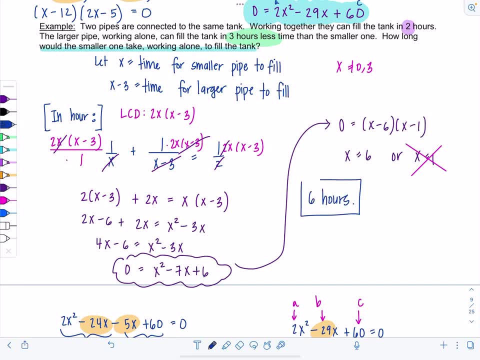 one would take six hours by its lonesome. Okay, We answered the question. Do you feel victorious? No, So we have to practice that you can do these effortlessly. It's like, um, I always say this: If I watch gymnastics, which I love- I love watching gymnastics. I can watch it day and night. 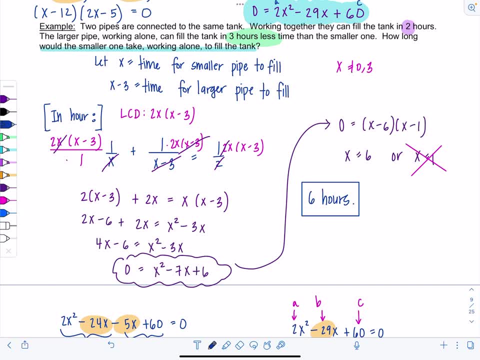 but it doesn't mean I'm going to be able to do anything impressive on the balance beam other than tumble off. It's only until you practice at something tirelessly that you too can do it effortlessly. Okay, And it's algebra. It's not as bad as gymnastics, I know it might seem. 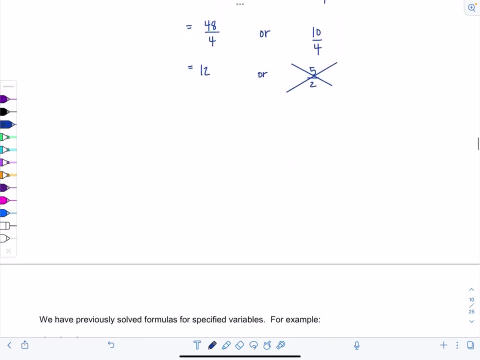 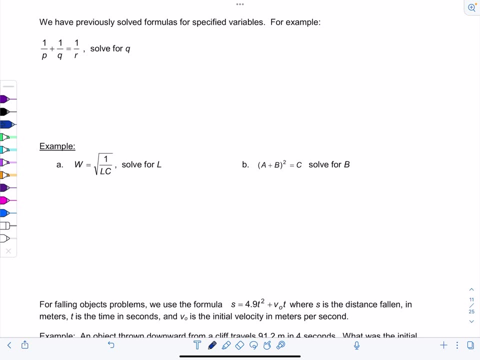 worse to some of you, but it's really not. It's not Okay. All right, Let's change gears a little. Let's still look at some different kinds of equations. Um, we've previously solved formulas for specified variables, For example. 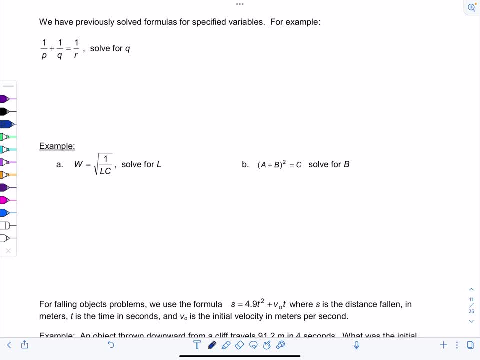 say: you have this rational equation and I ask you to solve for Q. What that means is you need to isolate Q, right? Whatever they ask you to solve for, you need to get that variable by itself. In this particular problem, since it's a rational equation, we would multiply by the LCD. 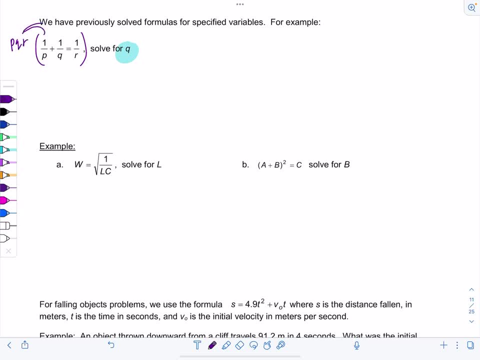 which is PQR plus PR to everybody. Okay, And then you would have QR plus PR equals PQ. This one's funky. What do you do when the variable you're solving for is in more than one place? Do you remember You want all those terms on the same side of the equation? 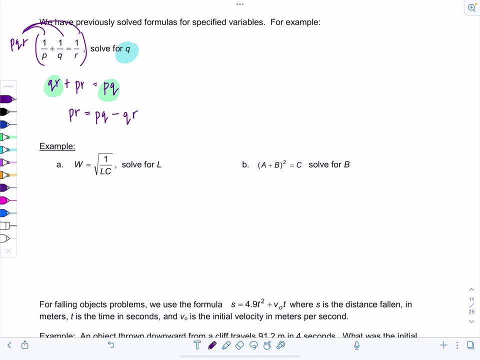 So I'm gonna leave PR over here and then let's get everybody who has a Q together. They want to be together, They want the Qs to hang on out. yes, and then we're going to factor it out. okay, so pr equals q times p minus r. and then now 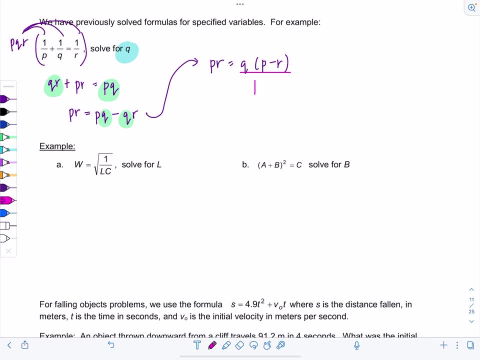 just divide by p minus r and you've got q by itself. do you see that we've done this before? being able to solve for a variable with this technique is very important. oh my goodness, you're going to have to do it throughout your math career. you're going to have to do it in. 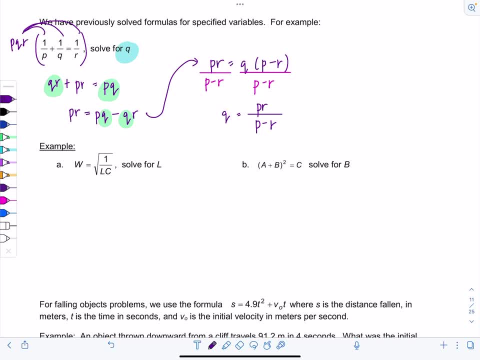 precalc. when you find inverse functions, you're going to have to do it in calc one. when you apply implicit differentiation and you solve for y prime, so being able to recognize- ah, i'm solving for q, it's in more than one place, put them together and factor it out, if you remember that. 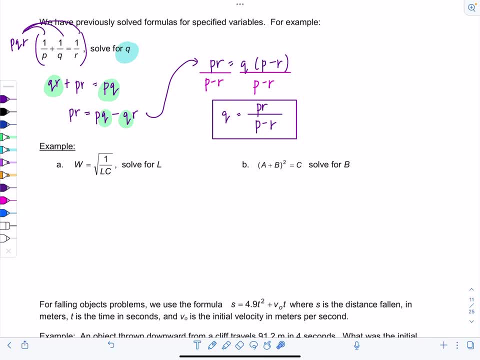 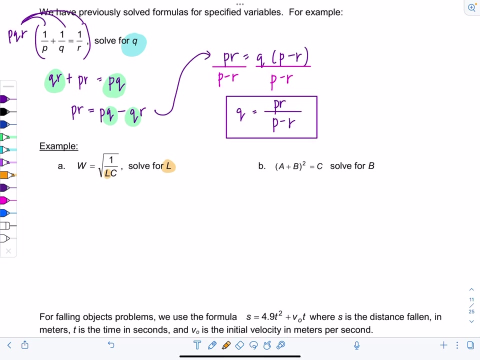 you're going places, okay, anyways, now we're going to deal with quadratic equations or equations with square roots and solving for variables. so same idea. say: you're given this equation, don't worry about what it means, okay, solve for l, get l by itself. well, i'm looking. l is there in the denominator, under a square root of all places. 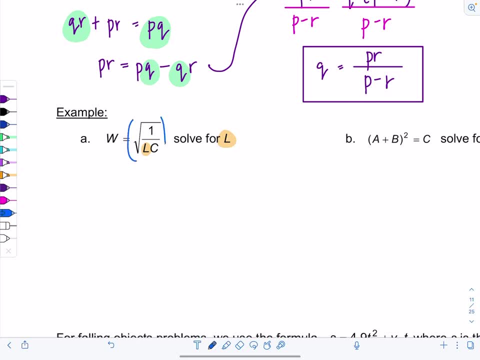 oh, what are you doing there? get out, okay. so let's square both sides, then we can get rid of the square root at least. so w equals one over lc from the hills. w squared. excuse me, okay, how do i get l out of the denominator? let's multiply everybody by lc. 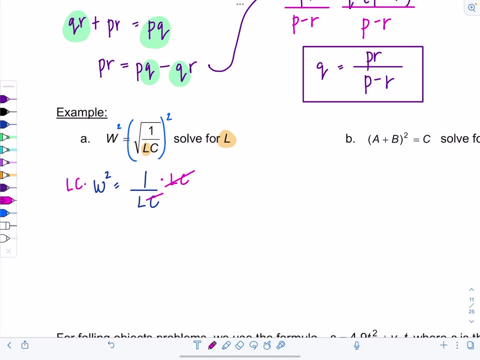 not more in comrade. okay, so we've got lc w squared equals one. who do i want by itself l? so divide by everybody who's bothering him? c and w squared be gone. okay. so that means l lc 8 plus l equal 1 over cw squared and we're done. okay, we're not going to get a number for our answer. 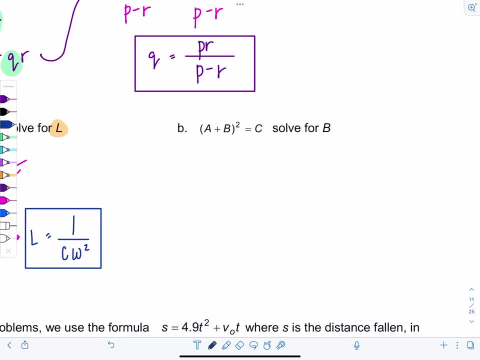 we're just solving for or isolating a variable. now next one solve for b. oh, a little different. b is inside these parentheses and that quantity is being squared. so what undoes raising something to the second power? how do you undo that? you take the square root right, but be careful, because we 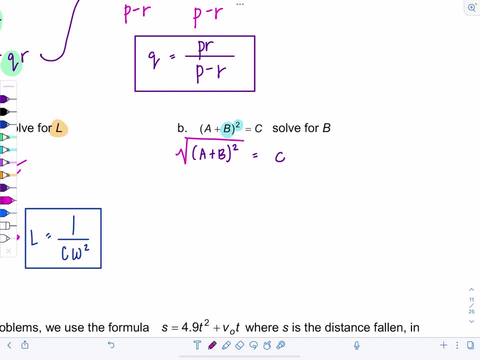 square root property which tells us when we take the square root of both sides of an equation. when we apply the square root, we have to put plus or minus. so then now I have a plus b over here, you don't need parentheses anymore. equals plus or minus square root of c. 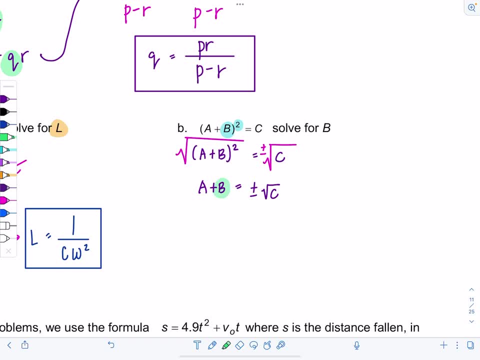 and then I'm trying to get b by itself, so this time I'm going to subtract a. they're not being multiplied, so don't divide by a, just subtract a, subtract a, and then that looks a little ugly. so the way we usually write our final answer is we would have negative a plus or minus rad c. 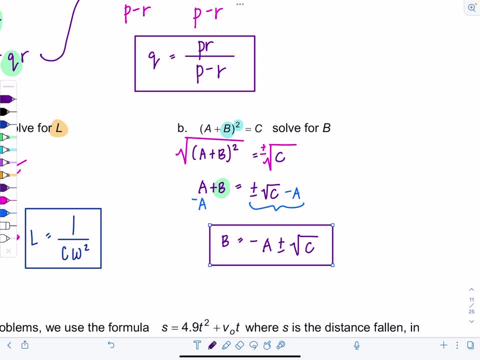 kind of similar to how we have it when we use the quadratic formula. right, you want that plus or minus square root part at the end? okay, I got one more problem for you. look at us. you probably were scared to watch this video and now you're grateful. 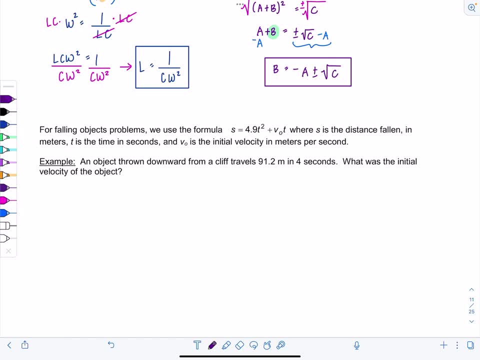 you're grateful. you're grateful. I hope now you'll see this more in physics later, should you take some physics classes. for falling objects we use the formula: s equals 4.9 t squared plus v naught times t, and I'm going to explain what all these variables are in just a hot second. 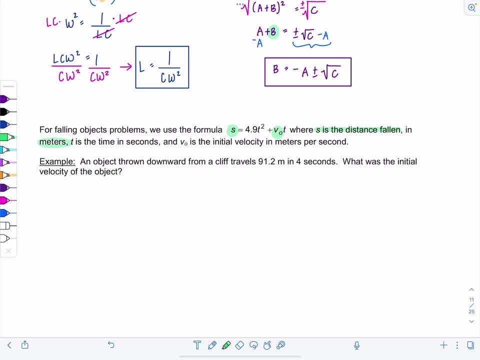 so s is the distance fallen in meters? yes, we use metric, t is time in seconds. that's kind of common sense. and then v naught is the initial velocity in meters per second. okay, so that little zero subscript means initial starting velocity. so let's do one little example: an object thrown downward from a cliff travels 91.2 meters. 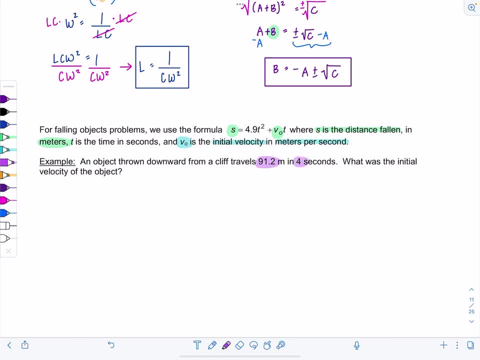 in four seconds. what was the initial velocity of the object? so 91.2, that's the distance s four seconds, that's t, and they want the initial velocity. so they want v naught. okay, so let's substitute everything into the formula s equals 4.9t squared plus v naught times t. 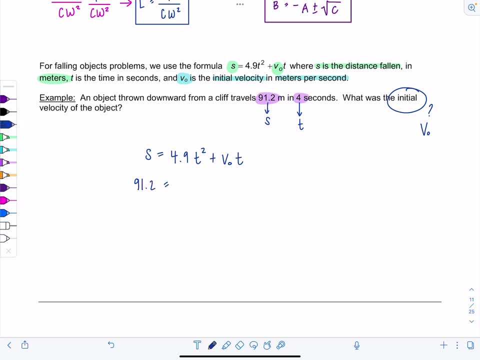 so s is 91.2. I don't put units in the equation. your physics teacher may want you to, though. okay, but in math I just don't like it. it looks messy. um equals 4.9Then how many units? um equals 4.9Txv0. but your quiz teacher is gonna DB. 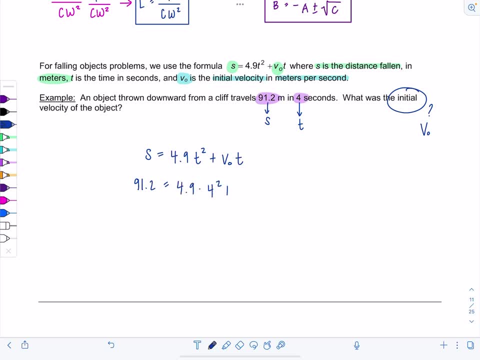 um, equals 4.9Txv0. but your physics teacher is gonna DB times 4 squared, plus V naught times 4.. So this is 91.2 equals 4.9 times 16, right, Perhaps I needed more parentheses like this: plus 4, V naught 4.9 times 16, that's 78.4..